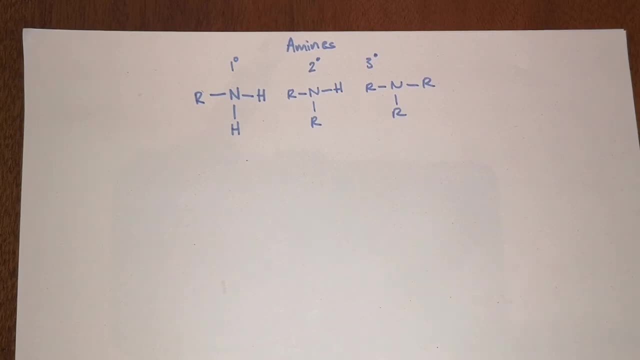 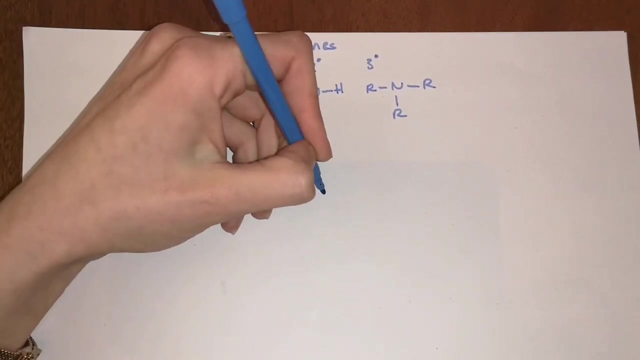 about then Is: what are the shapes of amines? So we briefly spoke about this already in the last video, but just in terms of what it looks like with regards to its orbitals. So if you take this molecule here, So you have nitrogen attached to a CH3. 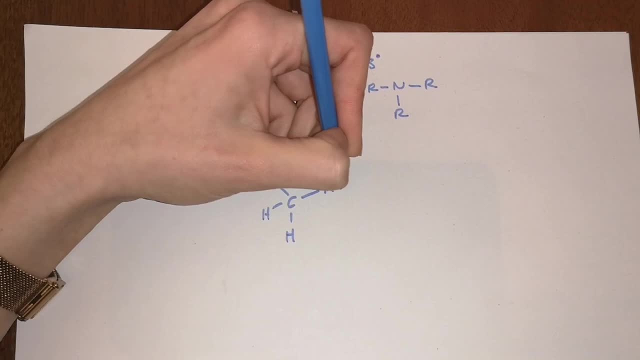 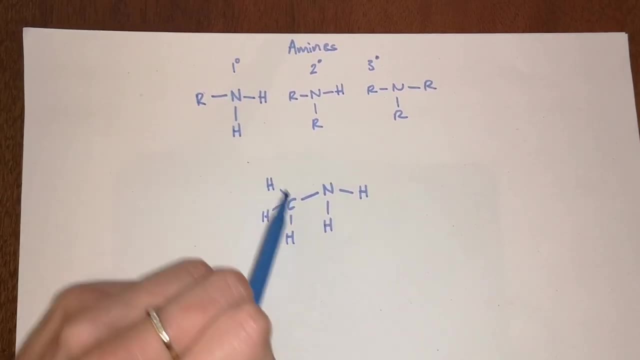 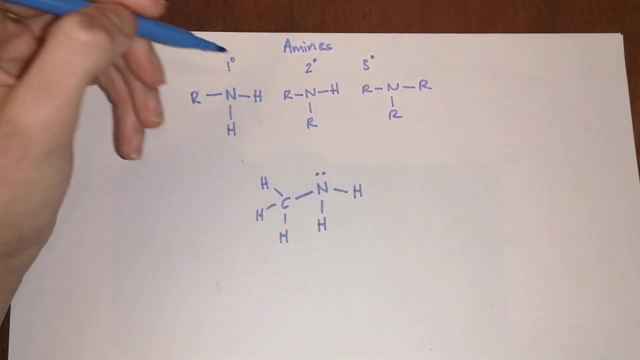 and there are two hydrogens as well, Okay. so in this case, hopefully, you're able to see that it's a primary amine, because it has one ore group, Okay, and then it also has a lone pair. So if you remember from the video on the shapes of molecules, you'll know that this is a pyramidal. 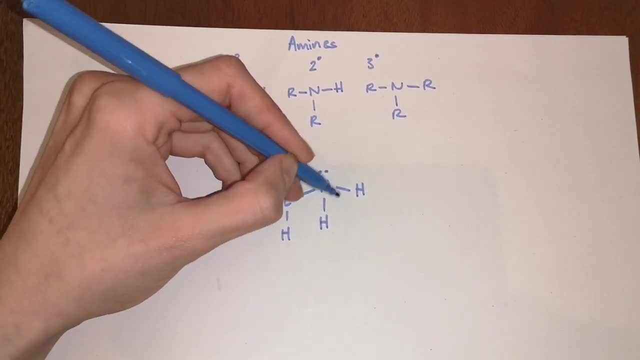 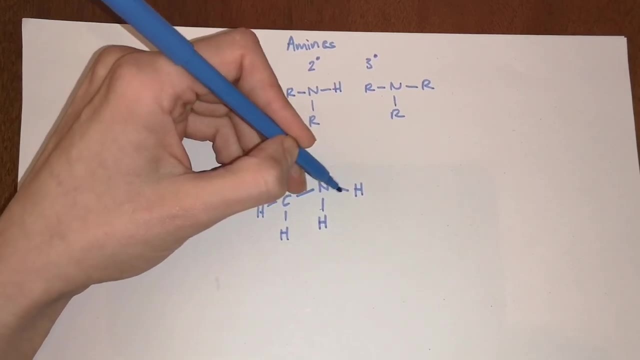 structure? Okay, because of the fact that it has four electron domains, much like a tetrahedral carbon such as in methane, But the lone pair repulsion is stronger than the bond pair repulsion, So the three bond pairs of electrons are pushed further down. Okay, so that's why it's pyramidal. 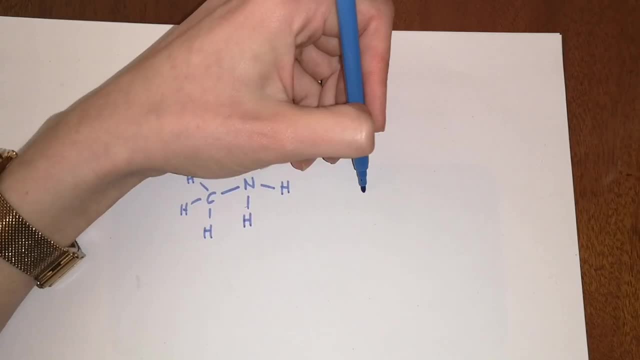 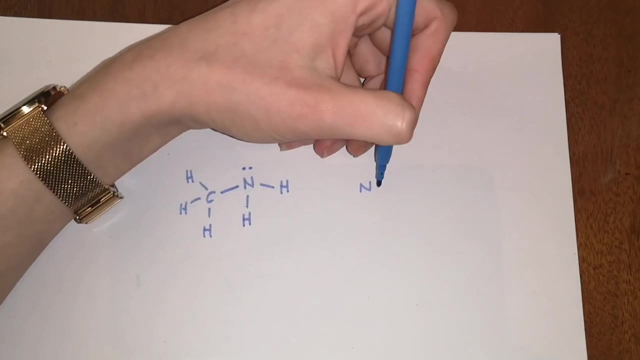 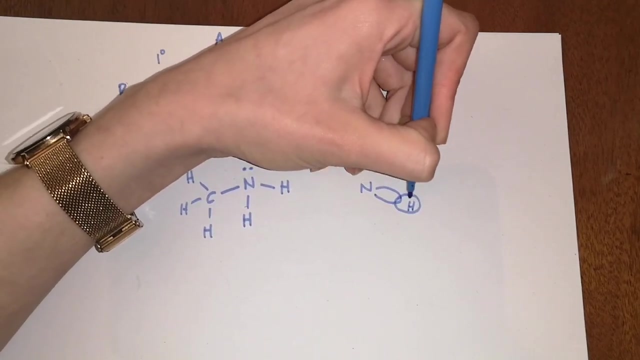 And in terms of what its orbitals look like: A primary amine or indeed a secondary, tertiary amine? These are going to be sp3 hybridized. Okay, so this is going to be similar to what we've seen before for methane. Okay, so if you have your 1s orbital of your hydrogen and then you have your sp3 orbitals, 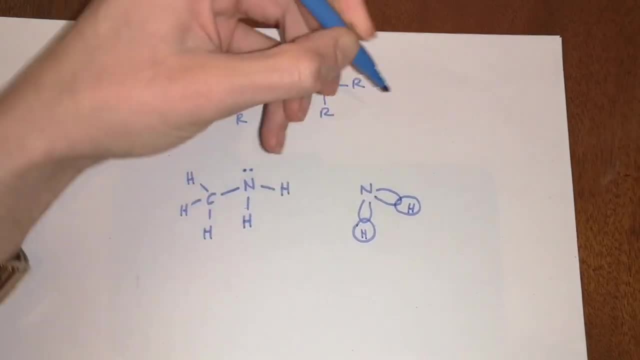 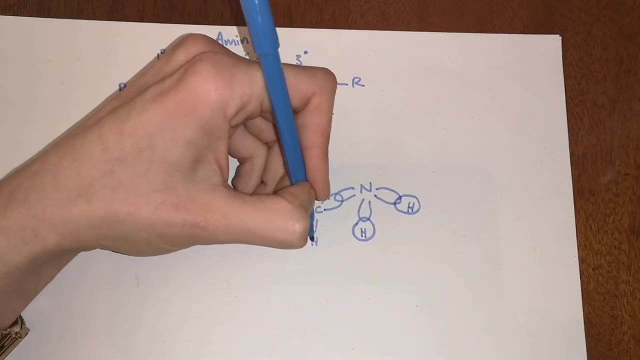 of your nitrogen, They overlap to form sigma bonds. So these are bonding orbitals. And then your carbon will also of course, have an sp3 orbital, And I'm not going to show them for these hydrogens, because they don't really matter too much. But then your lone pair of electrons. 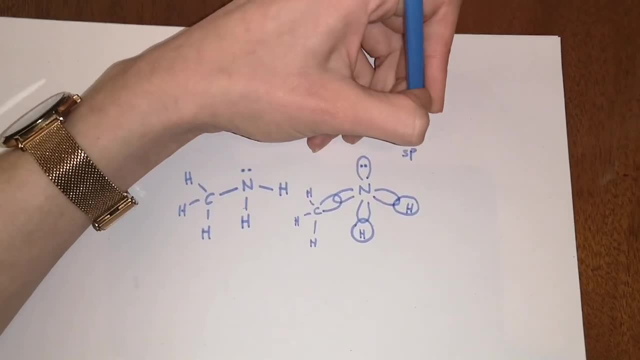 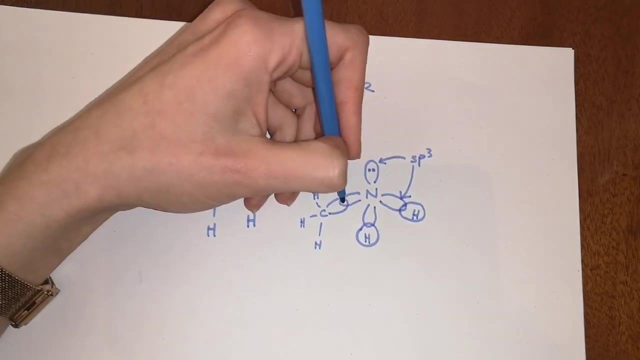 is also going to be sp3 hybridized. So this is going to be similar to what we've seen before for methane, Also in an orbital, Okay, in an sp3 orbitals. So what's important about being able to see this is what you'll notice- is that if you have your 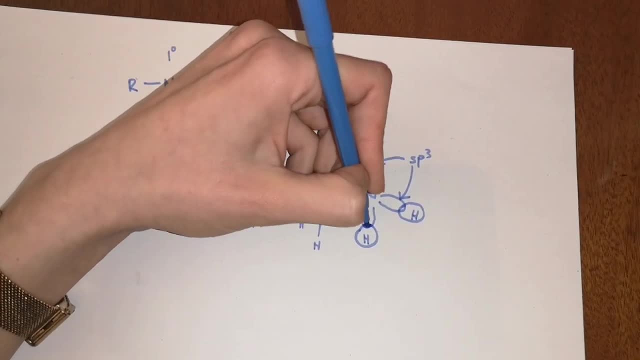 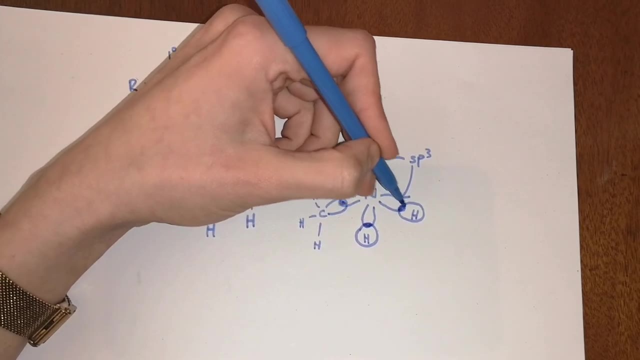 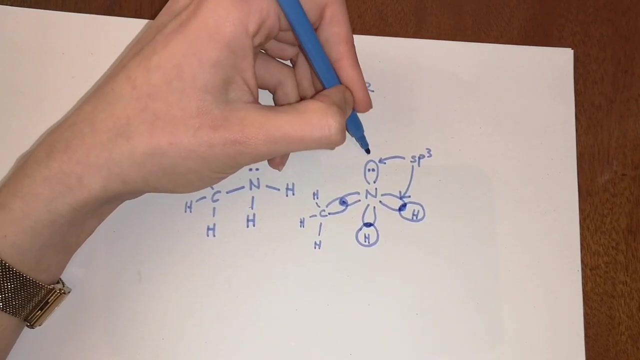 electrons in the bits where the orbitals overlap. Those electrons live between two nuclei And that means these electrons are relatively stable. When you compare it to this lone pair, it's only beside one nucleus. There is no other positive body here that stabilize this non-bonding nucleus. 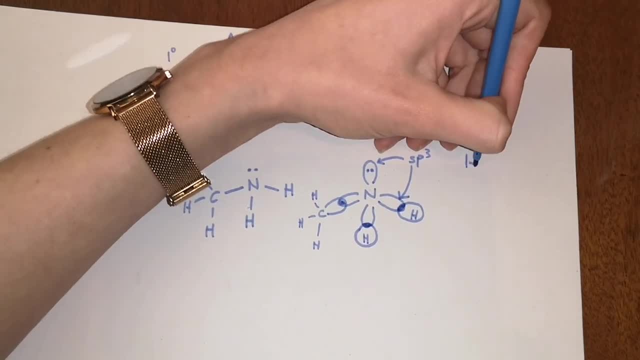 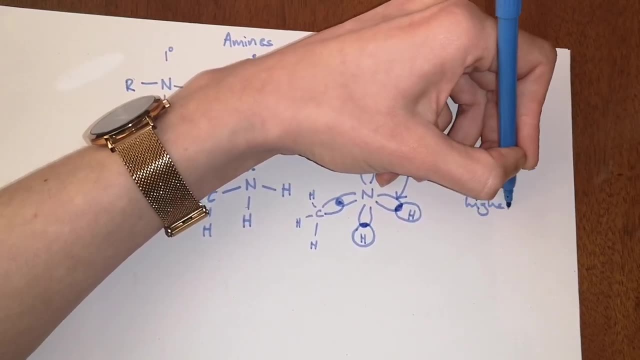 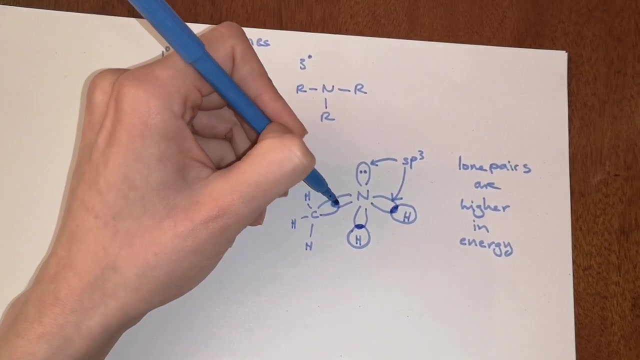 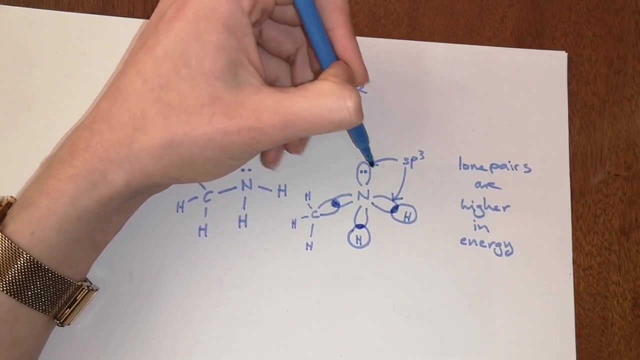 So this means that lone pairs are higher in energy And this becomes very, very important. So you will rarely see a sigma bond, The electrons in a sigma bond, attacking something else. But because the electrons in this non-bonding pair of electrons, this lone pair, Because they're higher in energy, they're quite reactive and they readily attack. 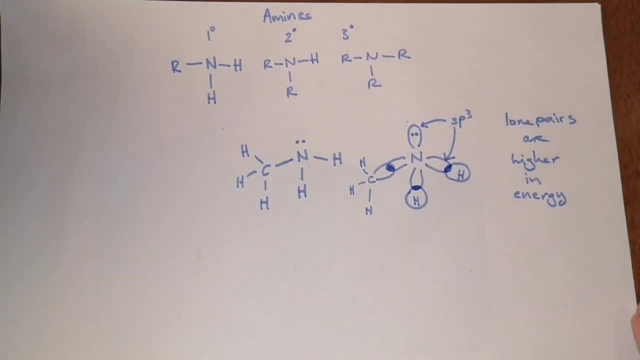 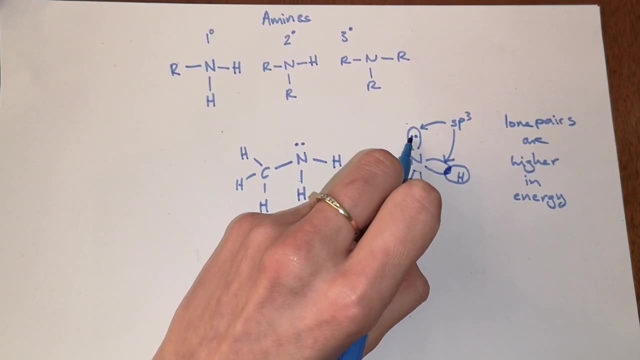 electrophiles. Okay, So from the terminology in the video where we talked about nucleophiles and electrophiles, Nitrogens are typically nucleophiles because of the fact that this lone pair of electrons is happy to attack a nucleus or something that's slightly positively charged, And because 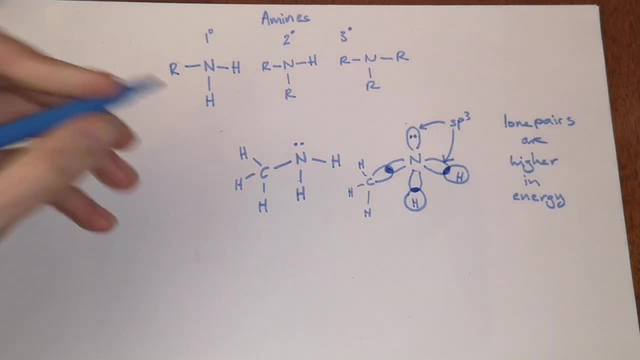 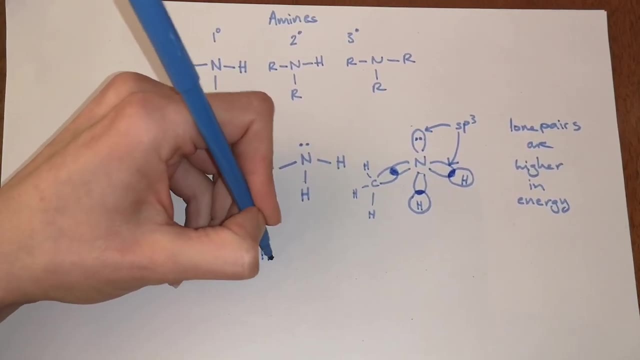 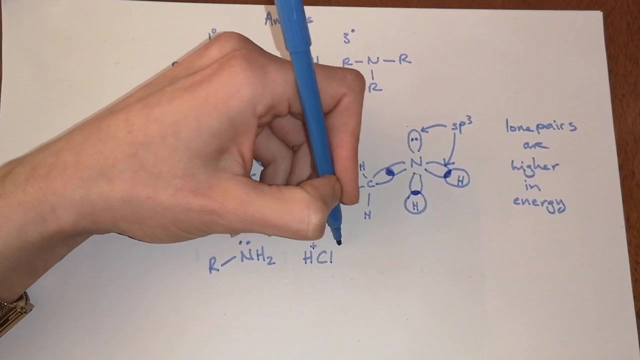 of that, it gives it quite a distinct reactive character. So amines, for example, are very good bases. So if you have NH2 like this and you have NH2 like this and you react it with, for example, HCl, okay, so it's H plus and Cl minus. 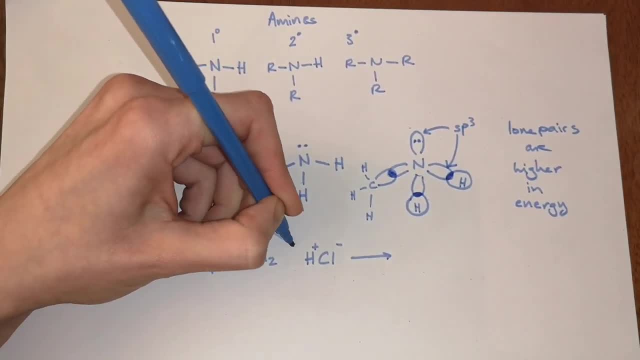 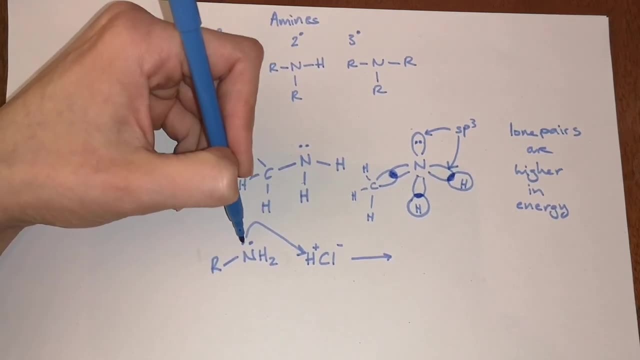 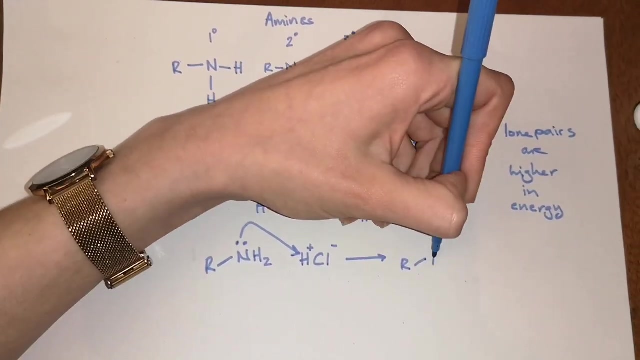 what happens is this lone pair will attack that hydrogen. and remember what we said about the curly arrow mechanisms. it's really important that the arrow starts exactly where the electrons are and it finishes at the atom you're forming a bond to. so now what you have is NH2 with an extra. 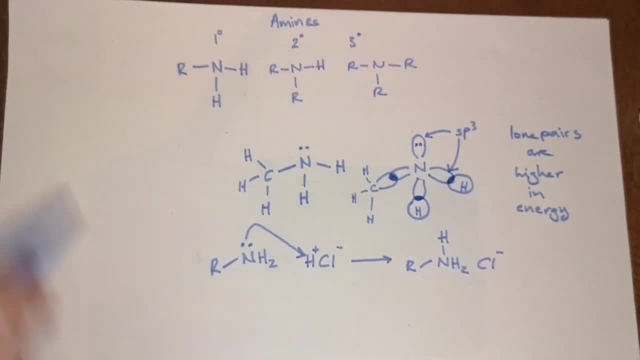 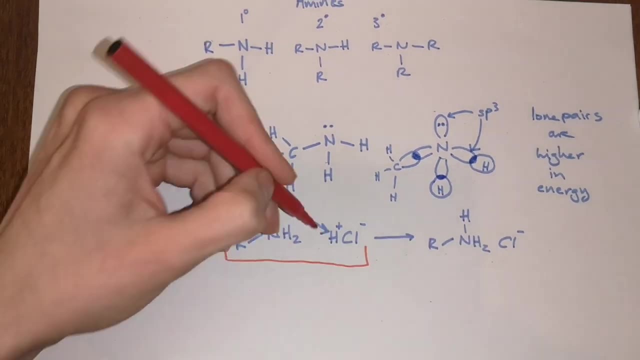 hydrogen on it, okay, and then you have Cl minus as well and, if you remember from the last video, what's really important is overall- sorry, I've scooted the page there. overall, this side of the molecule is neutral because you have one positive charge and one negative charge. so over here you. 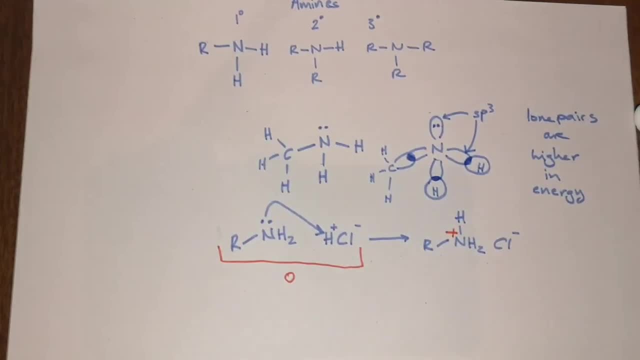 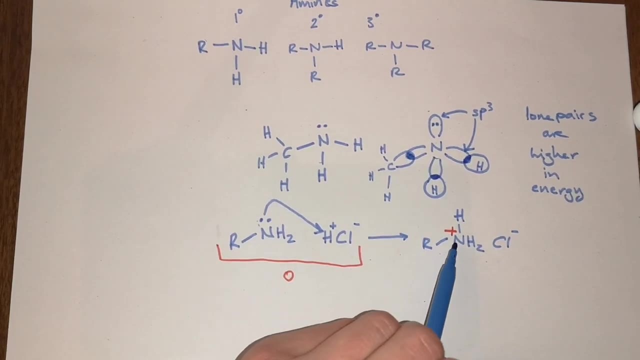 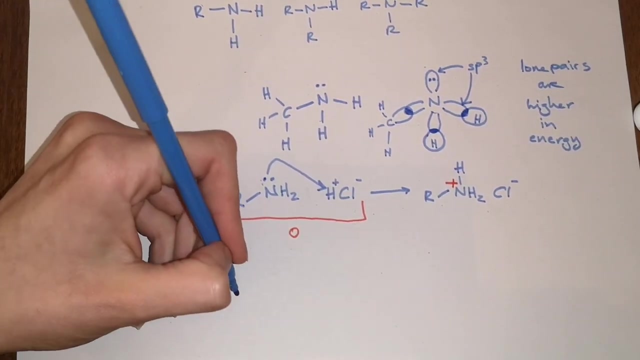 have your negative chlorine, but your nitrogen is now positively charged as well, okay. so if you have a neutral molecule and it picks up a proton from somewhere else, then that's going to be positively charged, okay. another aspect of the reactivity of amines is not just that they're basic, but also that they're nucleophilic. 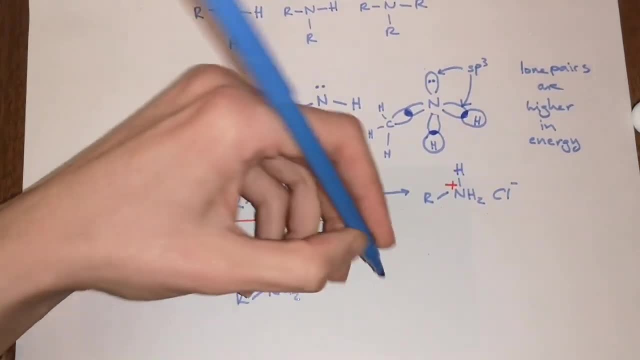 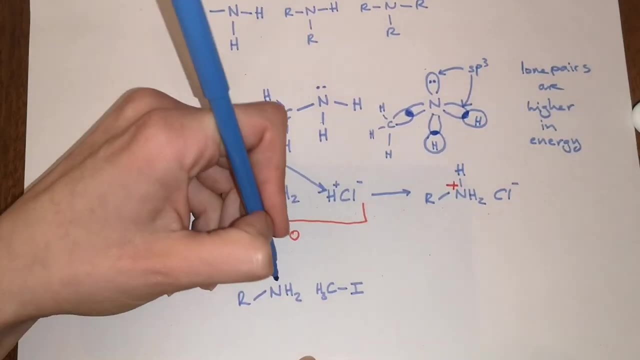 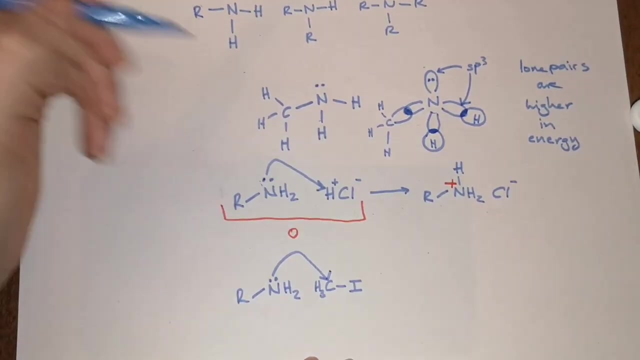 so if you have your NH2 like this and you take methyl iodide, okay, this lone pair, much the same as up here, this lone pair will attack this carbon and because carbon cannot have five bonds, as you attack this carbon, this carbon iodine bond will break. 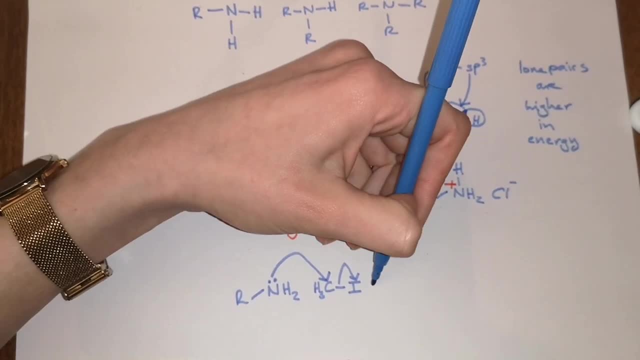 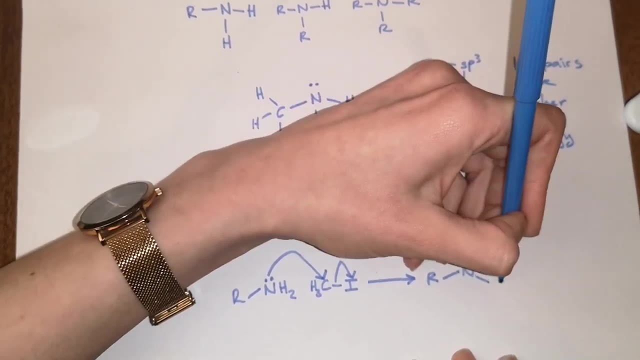 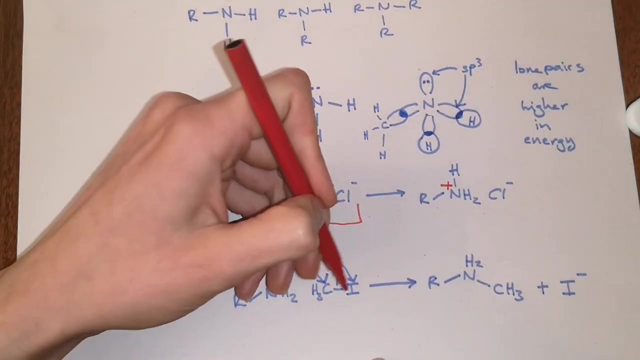 and the reason for that is because iodine is a very good leaving group. so then what you end up with is or NH2, CH3 plus I minus. okay, and it's important that you notice that it's I minus, because it used to share these two electrons, but now it doesn't share the 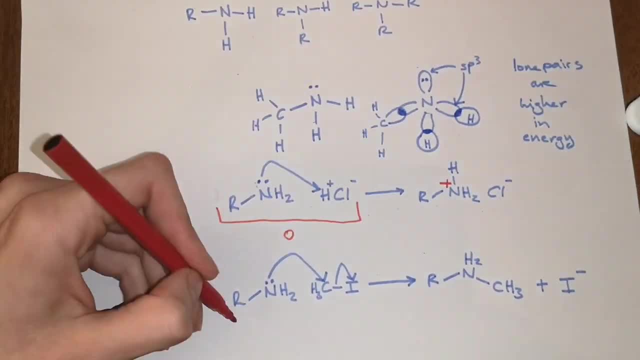 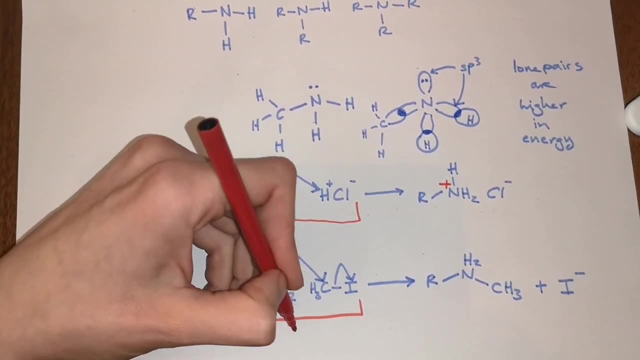 electrons, it has them both to itself. so it's negatively charged and same as before. when you look at this molecule, there's no. sorry, when you look at this molecule, there's no negative charge. on this side of the reaction there's no charges, so the overall charge is zero. and when you 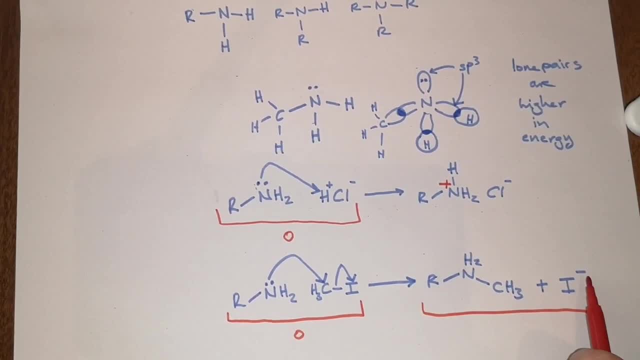 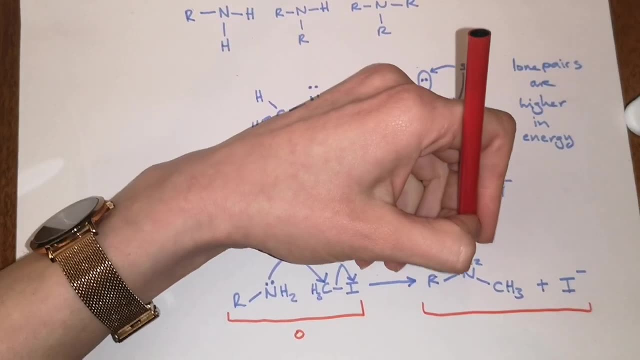 look at this side, currently it's minus one because you have one negative charge on your iodine. so you have to have a positive charge somewhere else to balance it and it's going to be over here with this nitrogen. so that's going to have a positive charge and the reason for. 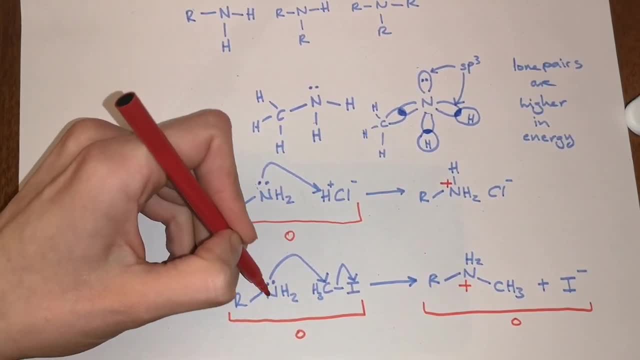 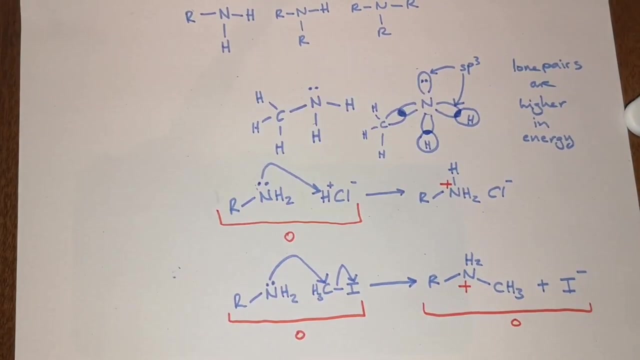 that is. this lone pair used to belong entirely to the nitrogen. okay, but when it forms this covalent bond, it's almost like it's donating an electron to the carbon. okay, so this lone pair, now it has joint custody, it doesn't have it all to itself, so it becomes 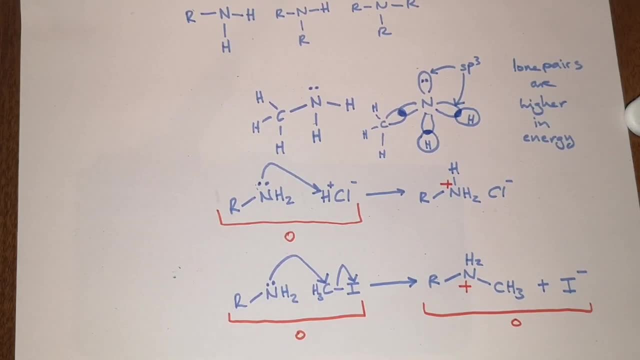 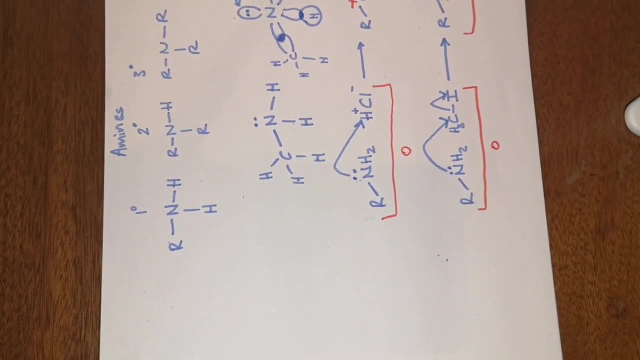 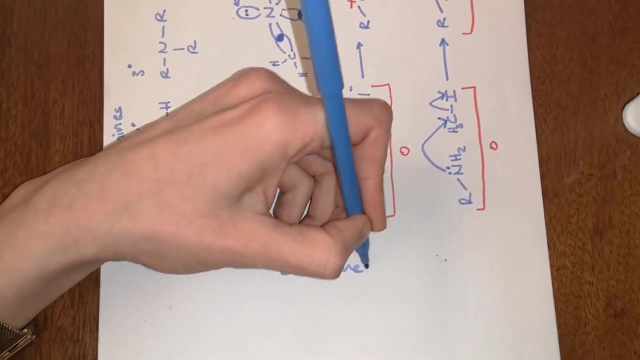 positively charged. the last important feature of amines- and I'm just going to turn the page sideways for this, save the trees- okay- is that the nitrogen hydrogen bond is polar. okay. so if we look at the electronegativity of nitrogen and hydrogen activity, if I spell that right, okay. 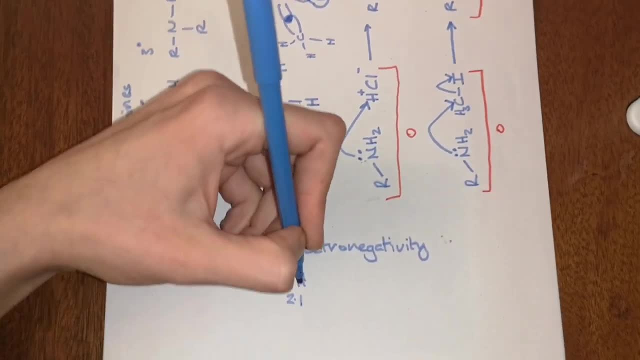 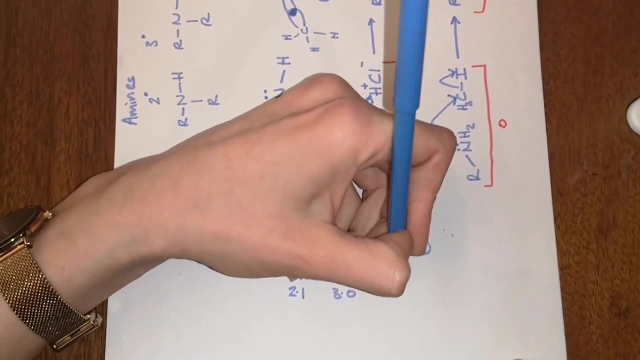 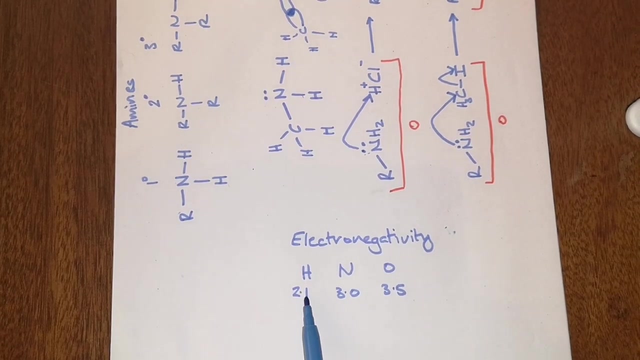 so hydrogen has a value of 2.1, nitrogen has a value of 3.0 and oxygen has a value of 3.5. okay, so the polarity in the bond of an nh is 0.9, but in comparison, if you compare it to an oh, it's 1.4. 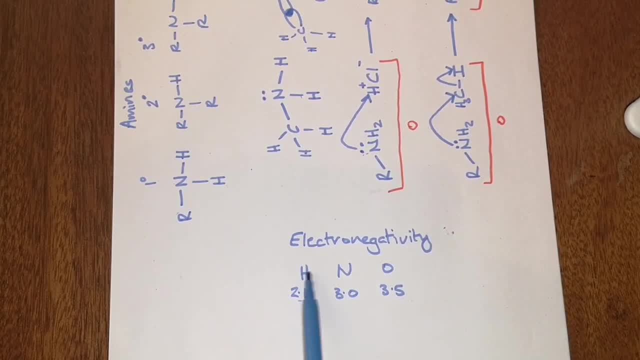 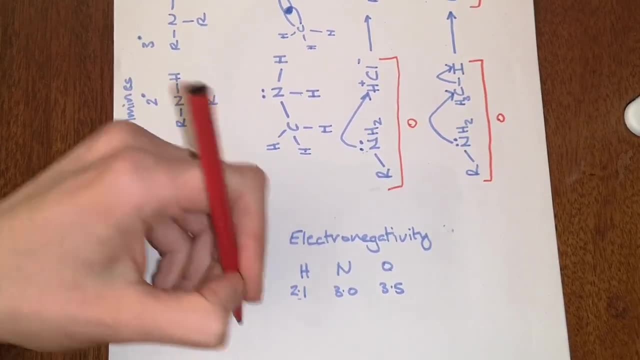 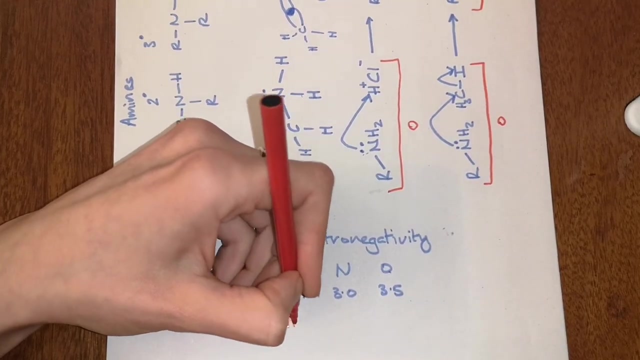 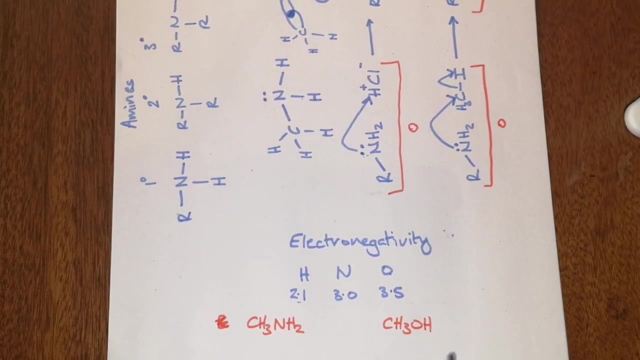 so the nh bond is polar, but it's not as polar as an oh, and this is very important, because what this is is if you compare- uh, we'll take a specific example. so if you take methyl amine and you compare that to methanol, okay, this hydrogen is more acidic because it's slightly more positively charged than these.